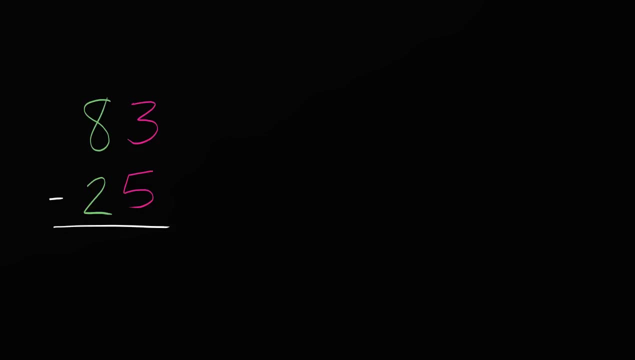 So how do you do that? Well, you could take a 10 from the tens place. So instead of having eight tens here, you could take one of them away, and then you're going to have seven tens here, And then if you take a 10,. 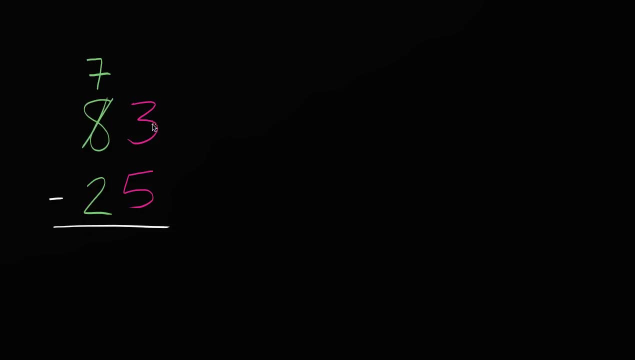 because I just took a 10 away from here and you put it in the ones place that's going to be 10.. So 10 plus three is 13.. 10 plus three is 13.. So what did I do again? 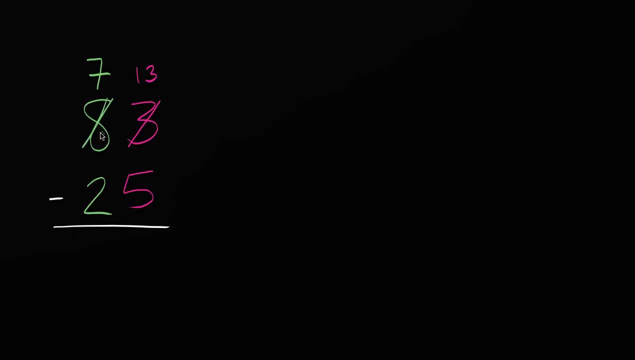 83 is eight tens and three ones. You could also think of it as seven tens and 13 ones, And I'm gonna do it again in a couple of different ways to make that clear. But let's just work through this now, Because now you have 13 ones minus five ones. 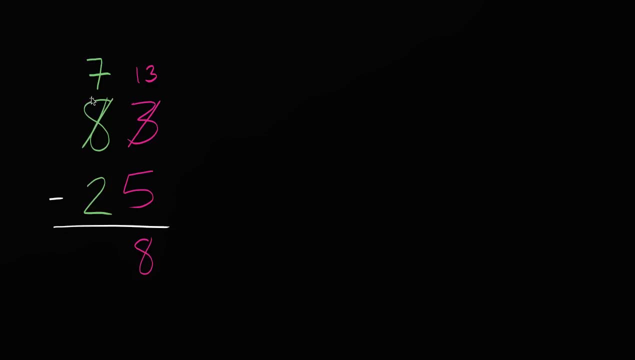 which is going to be eight ones. And then you go to the tens place and you say seven tens minus two tens. well, that's going to be five tens. So your answer is going to be five tens and eight ones, or 58.. 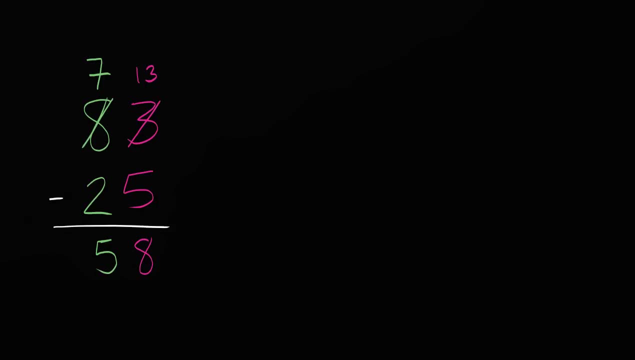 Now I said I would do this several ways so that it makes a little bit more sense. so let's do that. So another way that you could write 83 is you could write this: this is the same thing as 80 plus three. 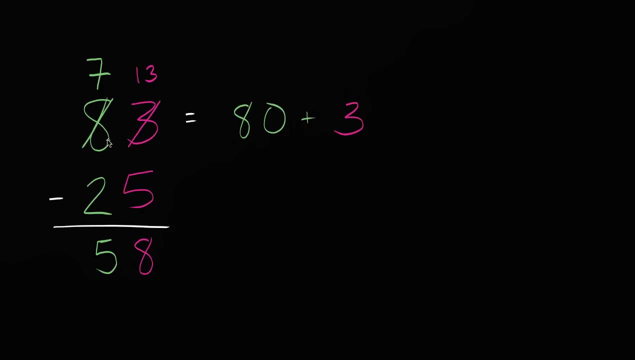 80 plus three, That's the same thing as 83.. Eight tens three ones. Eight tens three ones And 25 is the same thing, is the same thing as 20 plus five. 20 plus five. Now we're gonna subtract 20 plus five. 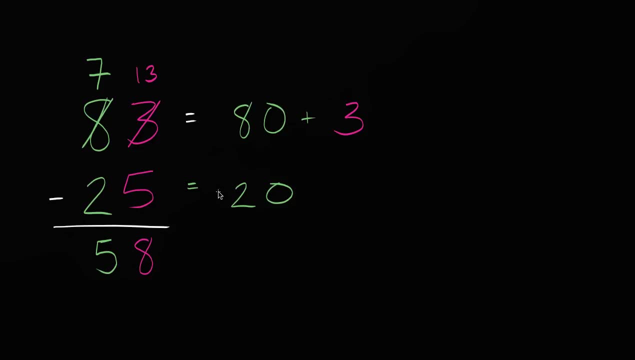 So let's write this instead, as we're gonna subtract 20,, we're gonna subtract two tens and we're going to subtract five ones. So subtracting 25 is the same thing as subtracting 20, and then subtracting five. 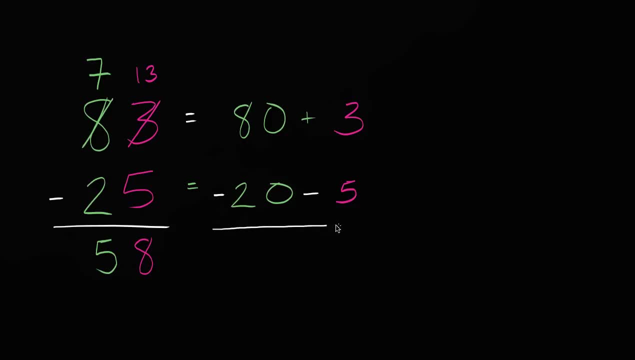 So now let's try to work through it, just like we did. Well, we go to the ones place again, and once again we say five. if I want to take five away from three, that's hard. I don't know how to do that just yet. 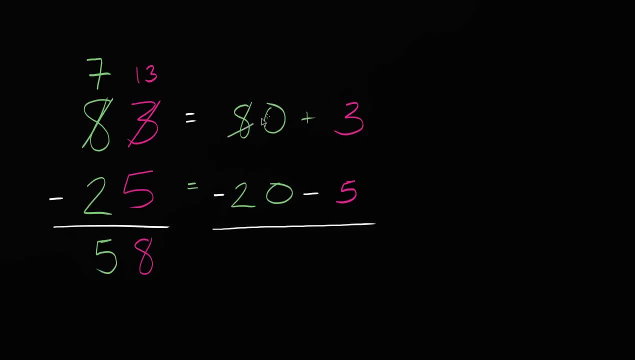 But what if I take 10 from here? So if I take a 10, if I take 10 from there, that's going to be 70. And if I put that 10 in the ones place, well, 10 plus three is going to be 13.. 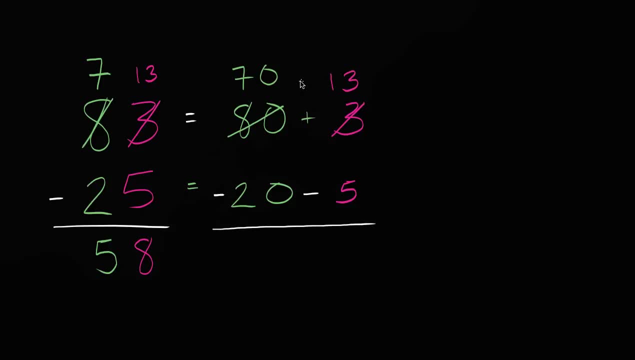 Notice I haven't changed the value of the number. 70 plus 13 is the exact same thing as 80 plus three, which is 83. But what's useful about this is now in the ones place I can subtract five from 13.. 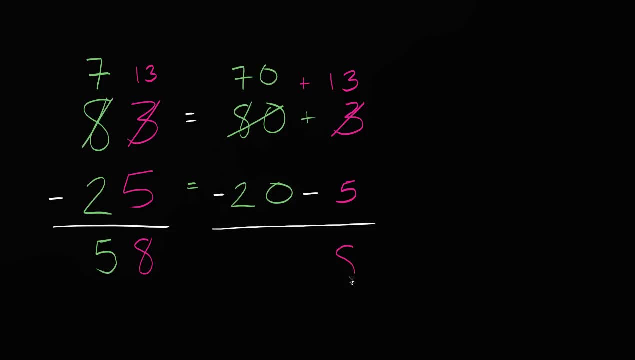 Well, if I subtract five from 13,, I'm gonna get an eight. And then if I subtract two tens from seven, tens, or 20 from 70,, I'm going to get 50. I'm going to get 50. So this is going to end up being 50 plus eight. 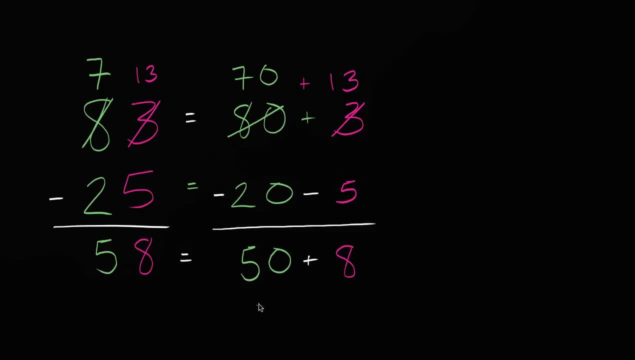 which is the exact same thing as 58.. Five tens and eight ones. Now I said I would do it a third way, And these are all the same way. I'm just writing it down in different ways. So I could also write 83,. 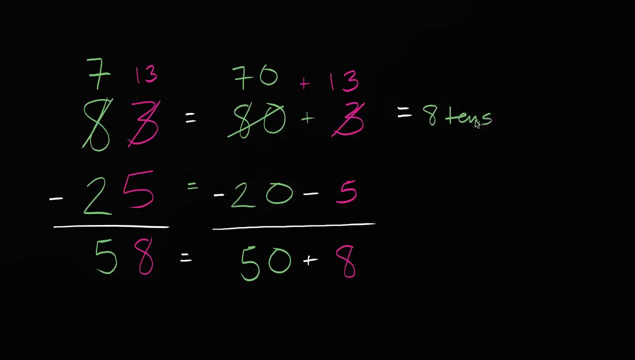 I could write this down as eight tens, eight tens plus three ones Plus three ones. Alright, this is the tens place, this is the ones place. Eight tens, three ones, And I'm gonna subtract two tens and five ones. So I could write: 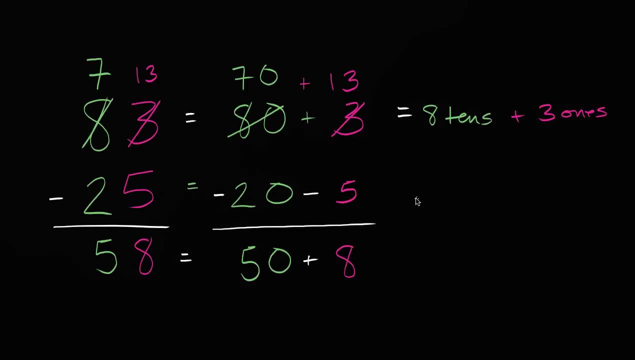 so this is going to be minus minus two tens. minus two tens and minus three ones, Sorry, and minus five ones. Minus five ones, 25 is the same thing as 20 and five If I'm subtracting 25,. 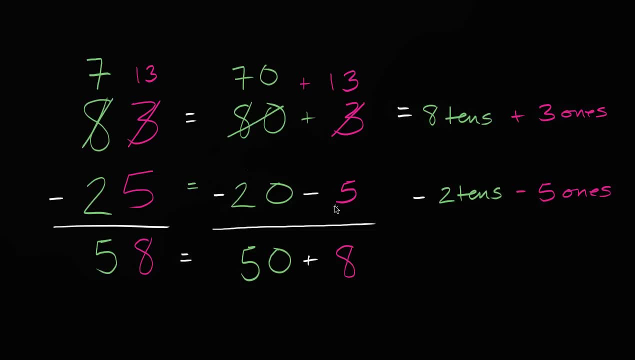 that's the same thing as subtracting 20.. And then subtracting five, And that's the same thing as subtracting two tens and then subtracting five ones. Two tens and five ones. So let's then work this out. So this is going to be. 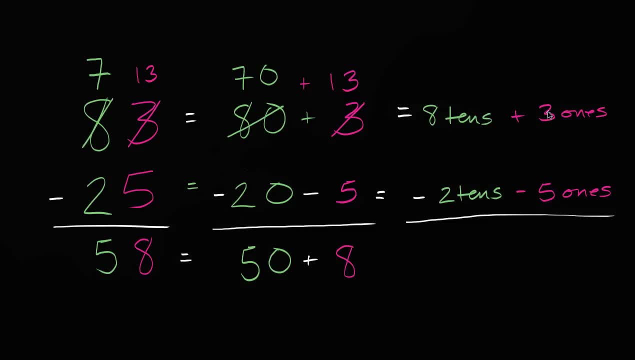 well, as soon as we try to subtract five ones from three ones, we say, hey, wait, that's not making any sense. Let me make the value here larger, And I'm gonna do that by regrouping from the tens place. 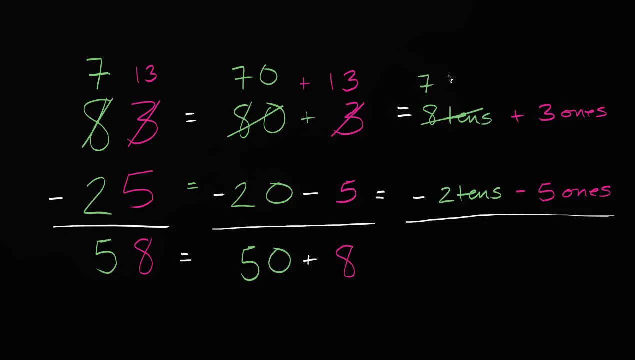 So instead of writing this as eight tens, I'm gonna take one of those tens away. I'm gonna write it as seven tens And then put that ten in the ones place. Well, one ten is equal to ten ones, So if I add it to the three,